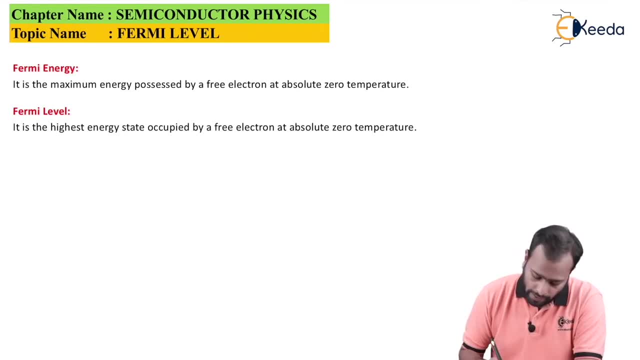 electron at absolute zero temperature. Well, in both of the cases you note that we are talking about absolute zero temperature. Zero temperature is nothing but as zero kelvin or minus 273 degrees centigrade. This is the temperature at which all the motion is seized. Now the important point to note is Fermi level. 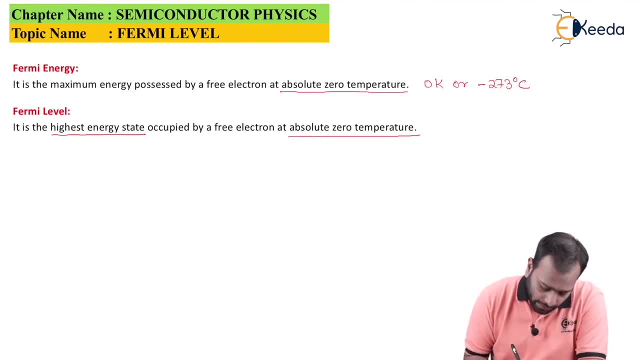 is the highest energy state and Fermi energy is the maximum energy possessed by free electron. So how would you basically distinguish between these two? Let's take an example of a material. This could be a metal, or any probable element or a substance. This is the energy state diagram. The green lines you can see are 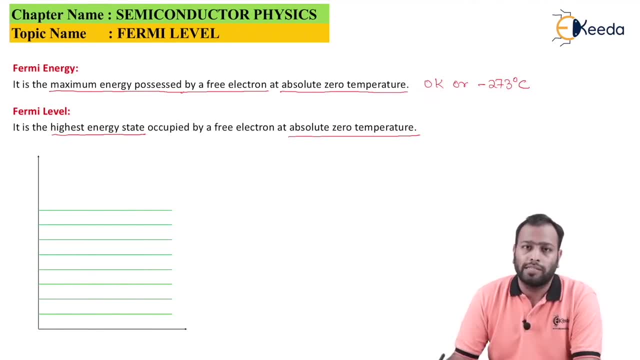 the various states of energy. Well, what are states of energy? Well, as of now, you just remember states of energy as regions, or particularly the hierarchy of energies, And these are the electrons. Now, if you look at the series you will find at this state, my last electron is: 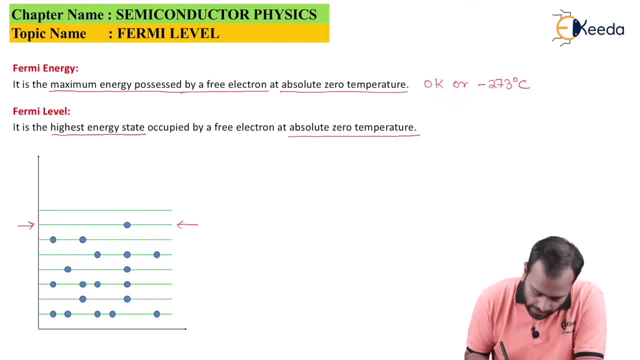 present, which makes this state as my Fermi level. Now, this could be clear by the definition. Now, Fermi level, it is the highest energy state occupied by a free electron. This is the free electron and the highest energy state occupied by this is the Fermi level. Now, if you look at the 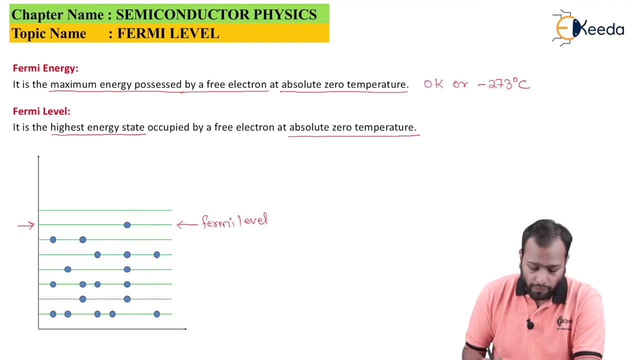 figure. so look at a specific的. this is a person who is speaking exactly with LED light. So this is a person who has a low energy state. So look at this. So basically, you can say that Fermi level is the highest energy state. 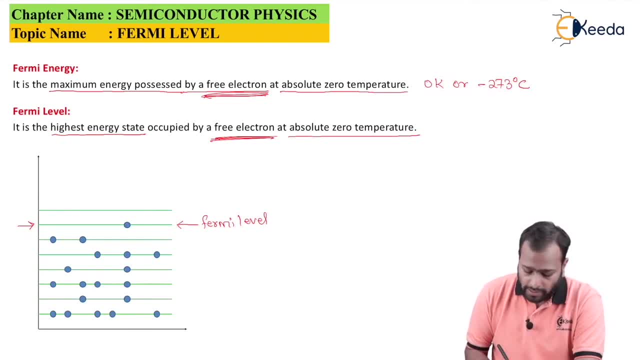 occupied by a free electron. So what exactly, for me, energy is then? Furmy energy is the maximum. could be easier to say that the electron at Fermi level, which is this electron, could possess the maximum energy. Is it always true? Well, no, There could be a possibility that this. 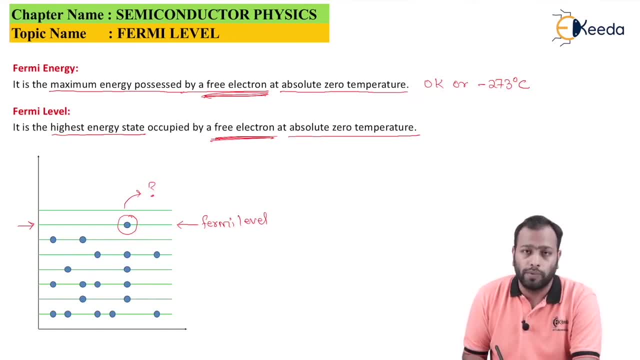 electron possesses maximum energy, but this is not always true. The maximum energy could be possessed by, let's say suppose, this electron. So the energy possessed by this electron will be called as Fermi energy. So Fermi level is the maximum state at which the free electron 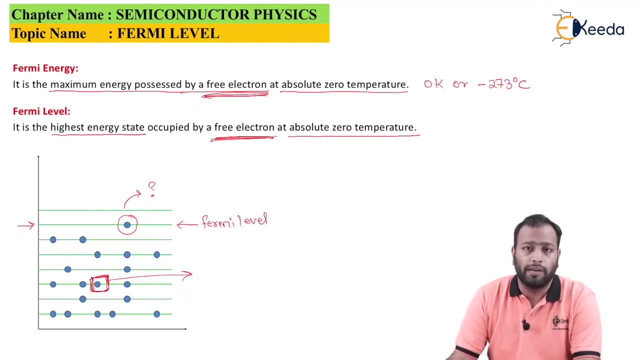 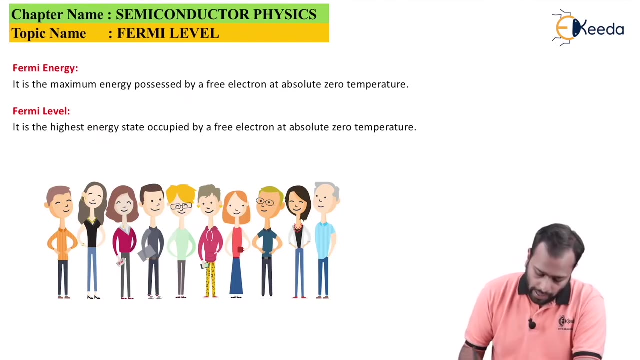 occupies, and Fermi energy is the maximum energy of any electron below the Fermi level. Now let's take a real life example and understand this concept very well. As you can see, there are people here, and among these people I elect this person as the Fermi level. So let's take 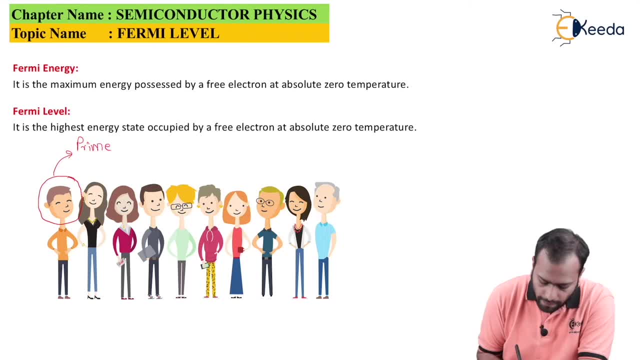 a�prime minister Now. so what you can say about them? well, you can say that this person holds the highest designation of any country, But is it necessary that he'll be the richest person in the country? Well, no, Let's say, suppose this person 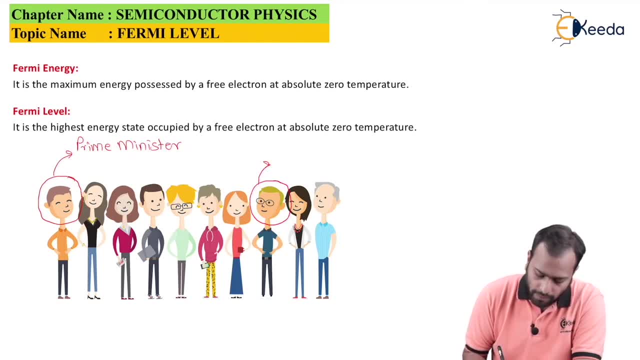 here is the richest man. he is the richest man of the country. now, this particularly makes clear about fermi energy and level. as you can see, prime minister is the highest designation or the highest state of any person in the country. so this actually represents fermi level and also this is the richest man, which 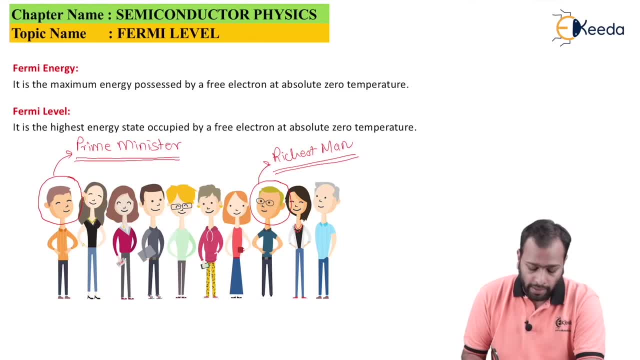 denotes the most powerful person in the country, and hence he represents fermi energy. so this is how fermi energy and fermi levels are distinguished. it's a very important point. you should make note, because this question could be asked as a viva question in your exams. now let's extend this. 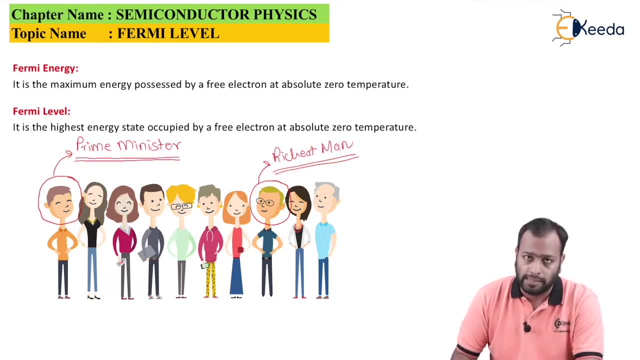 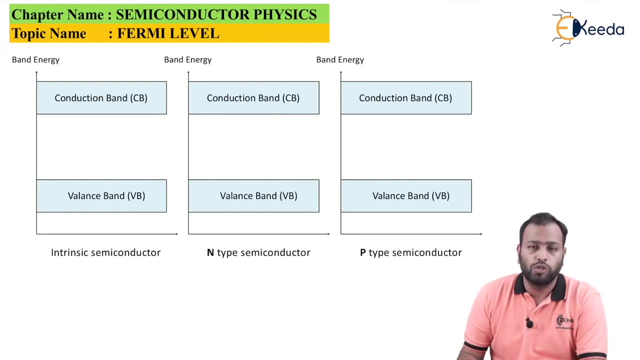 study to intrinsic and extrinsic types of semiconductor. now for an intrinsic semiconductor. we know that the valence band and the conduction band are the most powerful people in the country and hence he represents fermi energy. so this is how almost contains equal number of majority and minority carriers, which means that the number 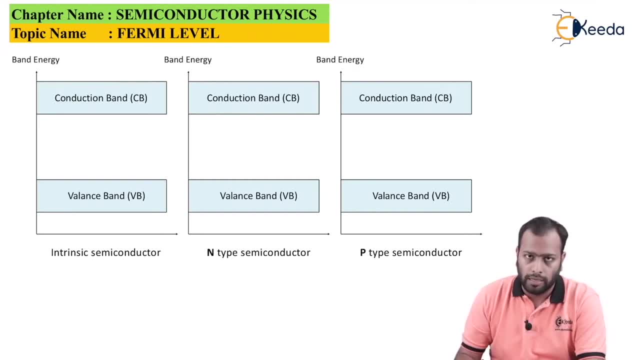 of electrons in the valence band will be equal to the number of electrons in the conduction band for an intrinsic semiconductor. the fermi level lies exactly at the center. this, so we'll call this as ef or the fermi level. now what happens in type of n type semiconductor? we all know that n type. 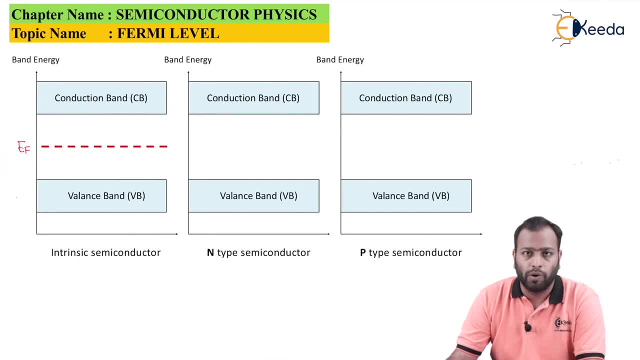 semiconductor is made by taking a pentavalent impurity into an intrinsic semiconductor. so if this n type semiconductor had been initially an intrinsic semiconductor, so of course this would be its fermi level. now, since there's an n type impurity or a pentavalent impurity added, which 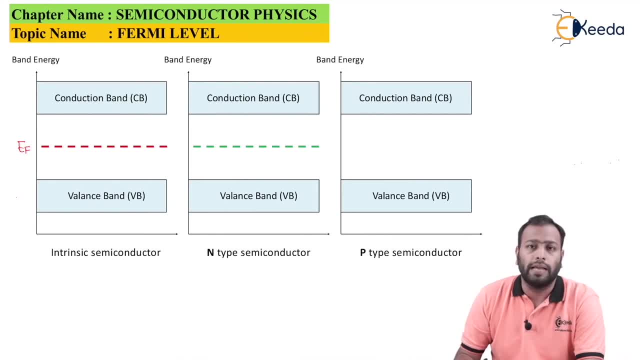 means that it has extra electrons, which again means that it has more number of electrons. so So the Fermi level shift towards the conduction band. So this is what the Fermi level is expected to be, But this is what the reality is: The Fermi level shift towards the conduction band. 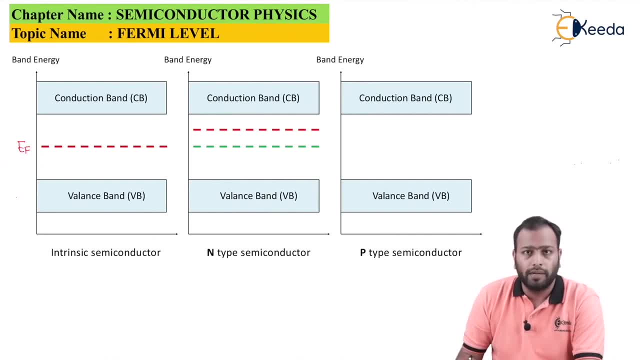 So well, it is now easy to guess what happens for the p-type semiconductor. We all know that in p-type semiconductor there is an electron deficient impurity which has been added, which is nothing but as a trivalent impurity. So if this had been an intrinsic semiconductor, this would be its Fermi level. 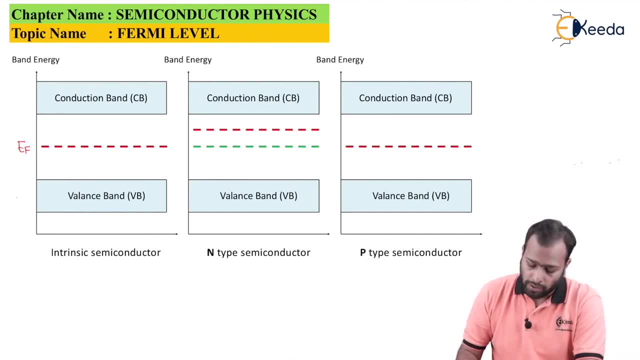 But since we have added a p-type impurity, so the Fermi level shifts downwards. So this is the Fermi level for n-type semiconductor And this is the Fermi level for p-type semiconductor. Now, well, as you saw, it is easy to say that in intrinsic. 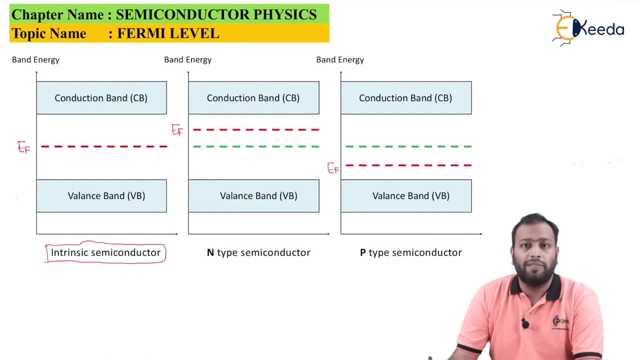 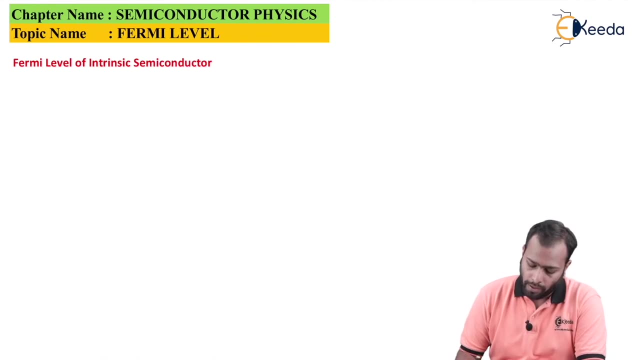 intrinsic semiconductor. the Fermi level lies exactly between the conduction band and valence band, But do we have a proof for it? Well, yes, This is the most important question for your university exams: Fermi level of intrinsic semiconductor. Now, let's recall. this is the band energy diagram for intrinsic semiconductor. 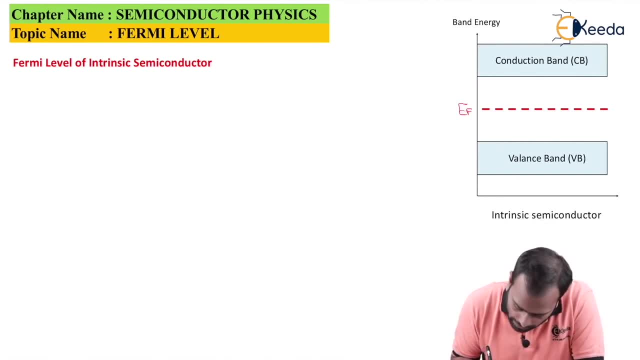 This is the Fermi level And this becomes my eV, The energy of the valence band, And this becomes the energy of conduction band. Well, the notations are very important. Ec stands for energy of the conduction band and eV stands the energy of the valence band. 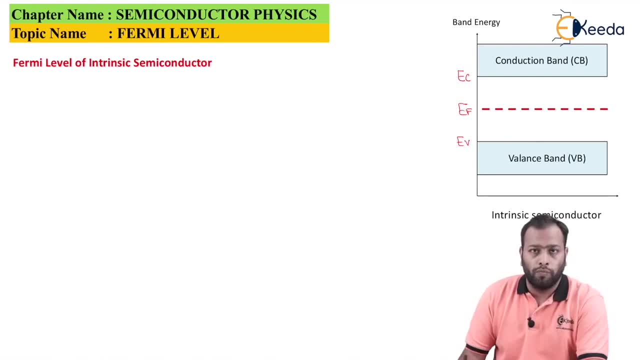 Ef, of course, is the Fermi level energy. We know that the number of electrons in the conduction band are given as: ne is equals to nc into e raised to minus e, c minus ef upon kt, Whereas the number of holes In the valence band is equal to nv e to the power minus ef, minus ev upon kt. 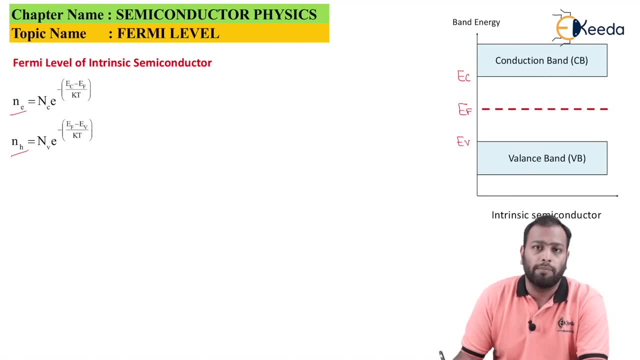 Ne and nh represents the number of electrons and number of holes in conduction band and valence band respectively, Whereas nc and nv represents the electron densities in conduction band and valence band. So important to know that there is a difference between small n and capital N. 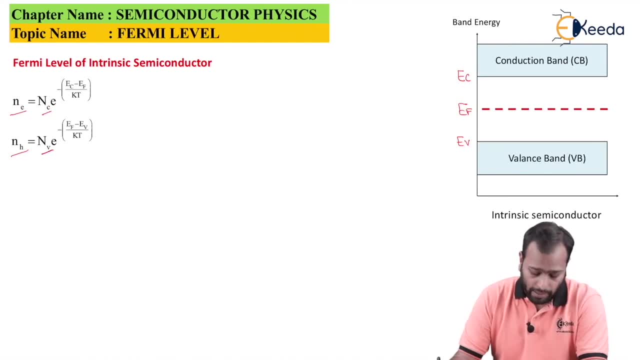 You don't need to worry about the values of capital Nc and capital Nv, because these are just the constants. But for better approximation we will be saying that nc is equal to nv. You have to make the statement before starting the derivation. 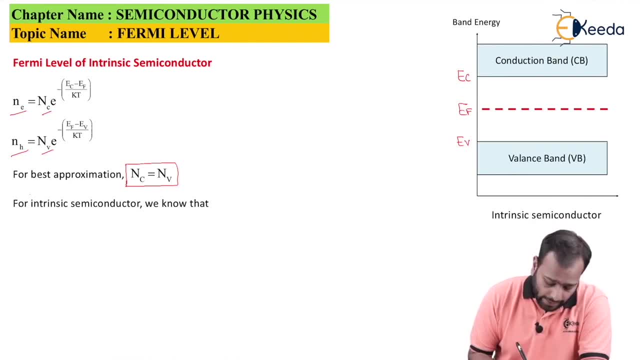 For an intrinsic semiconductor. we know that ne is equals to nh. or I can say that my number of electrons is equal to the number of holes. So if that is true, of course, the RHS will be true, So I can say that this equation holds true. 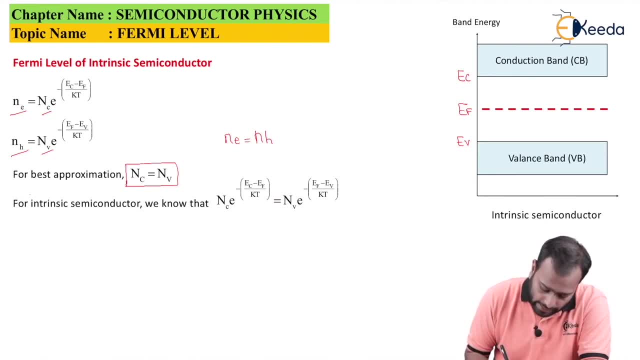 So well, if this is the case, I can cancel nc and nv from both of the sides for the better approximations assumption that I've already made, And the equation becomes this Now, as you can see, e to the power something is equal to e to the power something. 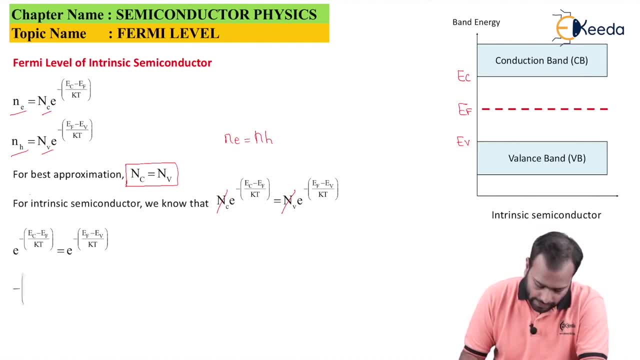 So of course both the things on the power side will be equal, Which makes minus of ec, minus ef upon kt equals to minus of ef upon ev upon kt. Canceling minuses on both the sides, and of course kt as well, will be getting this equation. 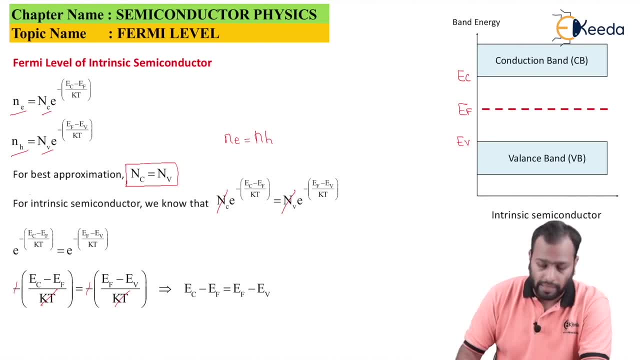 ec minus ef is equals to ef minus ev. Rearranging them would lead to: ec plus ev is equals to ef plus ef or nothing, but as ef is equals to ec plus ev by 2.. This is the important equation that we have derived, for, which means that in intrinsic semiconductor,